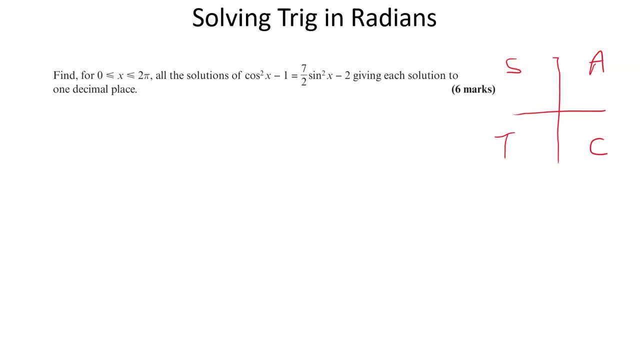 and then, depending on which ratio you're using, the other value will either be in this quadrant, this one or this one. So we'll come back to that. Let's look at this question in particular. It's got some squared cos and sine in it, so it looks like we're going to use the relationship. 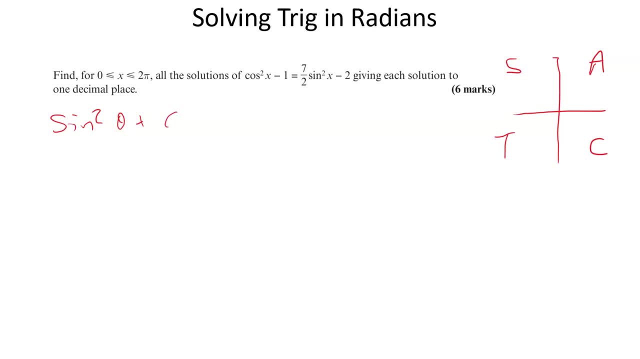 that sine squared theta plus cos squared theta equals 1.. And in fact they've already rearranged this to be cos minus 1.. So that looks very similar If I move the cos over here. if I took that away, then I'd get 1 minus cos. 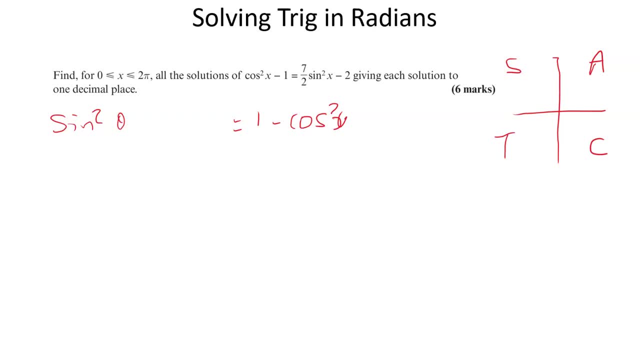 So that's almost what we want, but of course it's the other way around. So we can do that. We can just say: minus sine squared, theta is minus 1 plus cos, which is what we've got here: Cos squared minus 1, cos squared minus 1.. 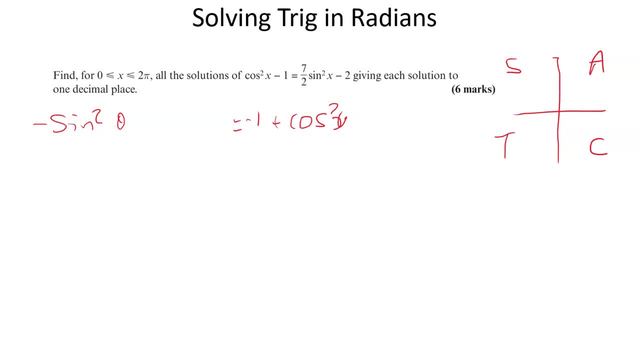 So we can rewrite this whole thing, but just replace this with minus sine squared theta. So let's do that down here: Minus sine squared theta Equals 7 halves sine squared. well, they're using x, not theta, but there we are. 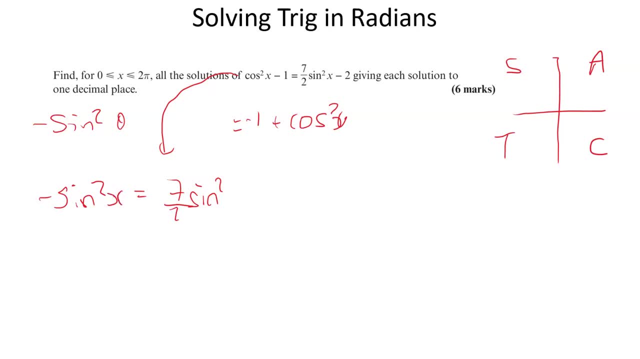 So x sine squared x minus 2.. So we can bring this all together and say: let's bring the 2 over and the sine over here. So we've got 2 equals 7, halves sine squared x, Plus sine squared x. 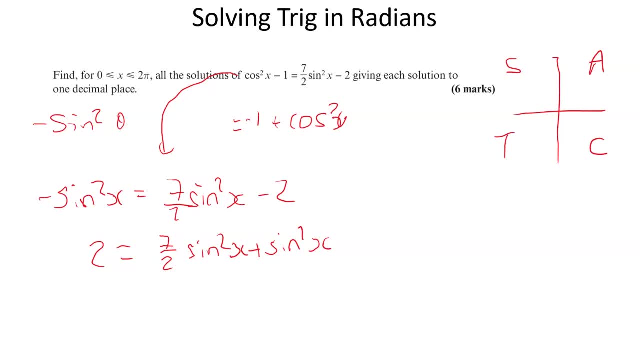 Just adding that over- And of course we can just group this together: 7 halves plus 1 whole 1 is going to be 9 halves. So we'll just add another whole 1 onto that and say it's 9 halves. 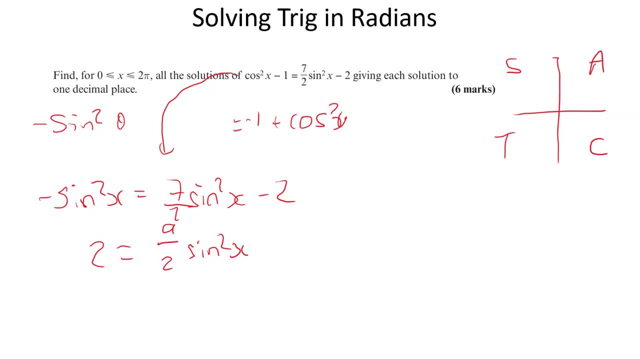 Got to get rid of this. so let's times by the 2,, divide by the 9, and say that sine squared x equals 4 ninths. We can then square Root that and get. let's come up slightly higher and get that sine x is the square root. 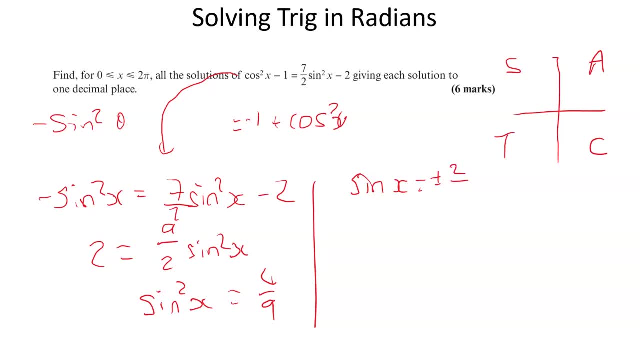 So it's actually plus or minus 2 thirds. So we're going to end up with potentially 4 answers here And then we can just do the inverse sine. So we need to do inverse sine of 2 thirds And see what that gives us. 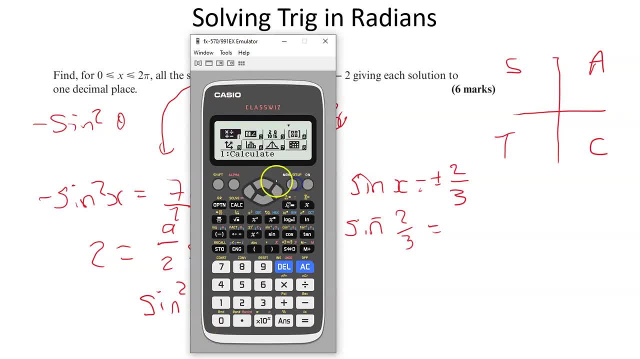 So, as we're in radians, make sure Our calculator goes into radians. So shift, set up angle unit radians, Shift, sine of 2 thirds And we get the answer of 0.729 or 0.730 if we round it. 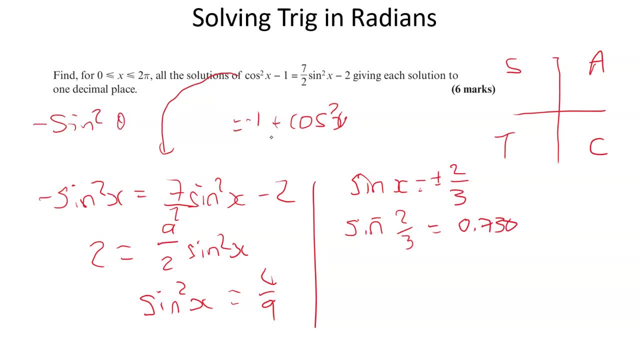 Now this gives it positive because it was giving positive 2 thirds. So This is giving it an angle here And this makes sense because this is less than half of pi. So the other place where we're going to get a positive value for sine. 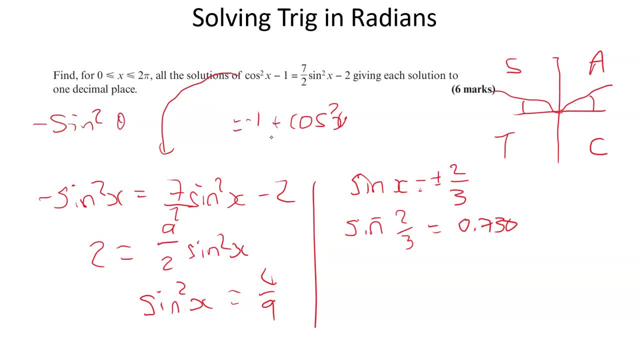 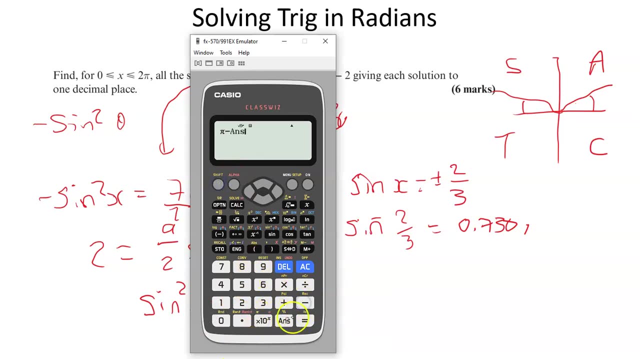 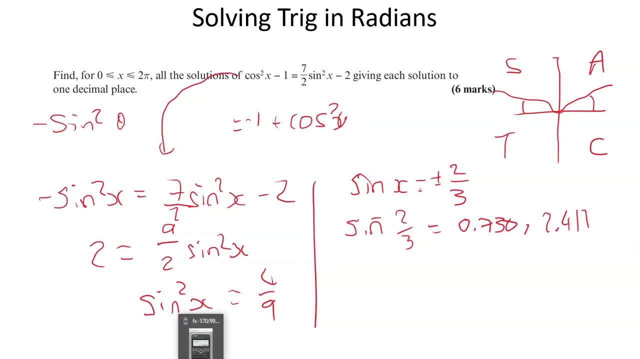 is on the other side, the same distance but away from pi. So to get the other value we're going to have to say what is pi minus that answer, And so the other correct answer should be 2.411.. Let me just check if that rounded. 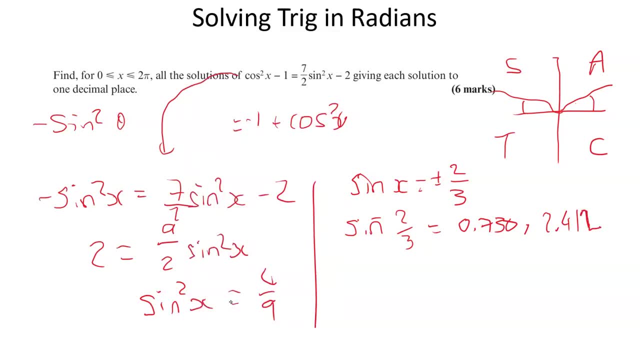 Oh yeah, a 2 at the end. Okay to round that, But of course we could also have done- sorry, I just realised- sine to the minus 1 there. We could also have done the inverse sine of the negative answer. 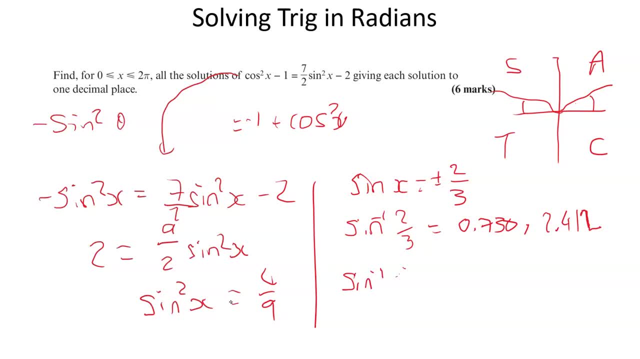 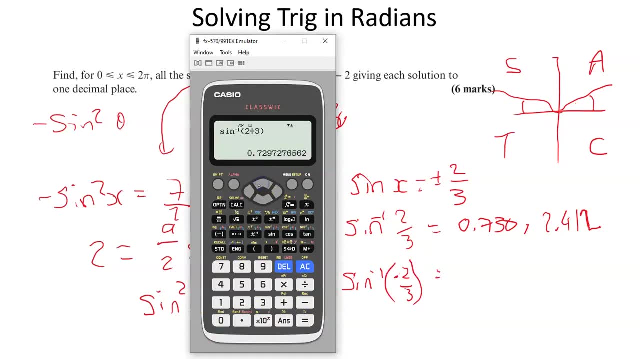 So sine to the minus 1 of minus 2 thirds. Okay, and let's see what that gives us. So go back up and put a minus sign on there And we've got minus 0.72. da, da, da, da da. 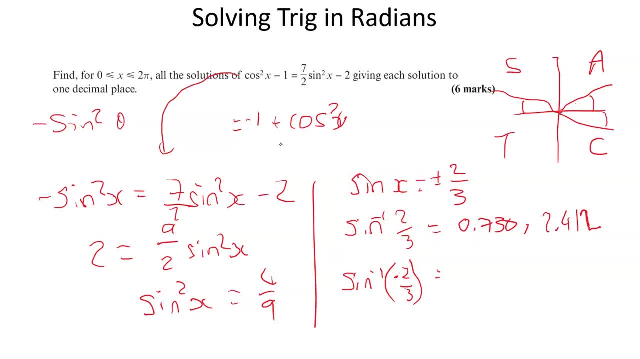 Which is? Which is the same amount as we had before, but underneath the axis. But we can't have that. We're going from 0 to pi, So we actually want the angle that goes all the way around to there rather than negatively down. 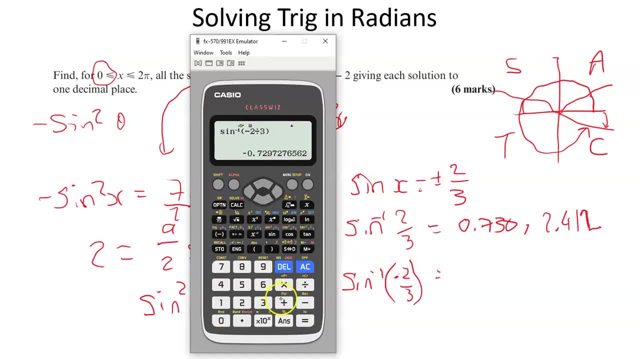 We need to go the correct way around. So what we want to do is just add a full circle onto that. So we add on 2 pi And that should give us the big angle all the way around. So this is 5.55.. 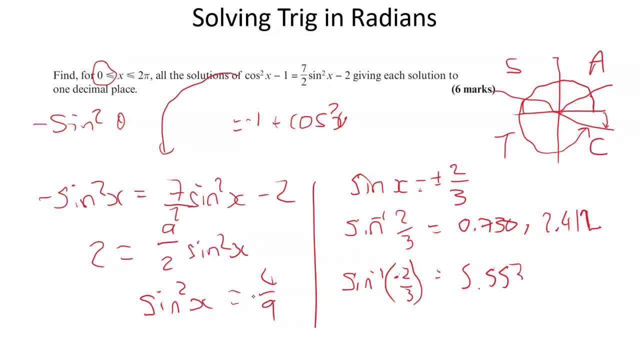 All right, let's put the 3 on. I seem to be doing it to three decimal places, not sig, fig, but it doesn't matter. So that's our first answer And because this sign gave us a minus answer, that's why we're in a in the C. 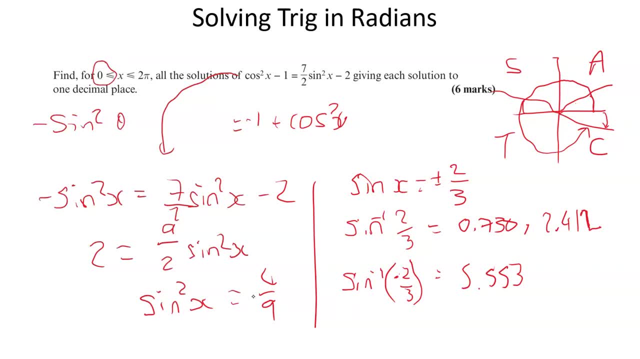 Yes, remember these letters tell you which trigonometric ratio gives a positive answer, in which, in which segment, not segment- in which Segment, Uh, quadrant of the of the graph. So all of them are positive here and sign is positive there. 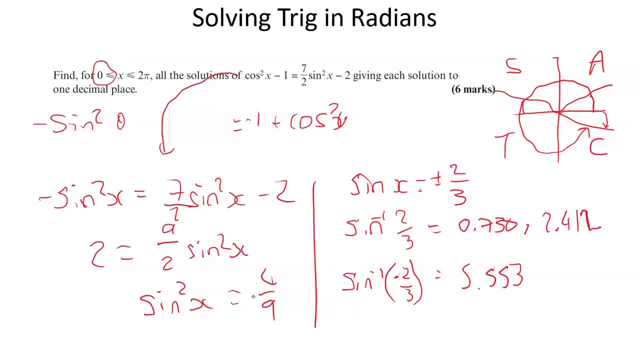 That's why we took our two positive values here. But this sign of X gave a minus two thirds means we need to be in the two quadrants which are negative for sign. Well, this is one of them and this is the other. 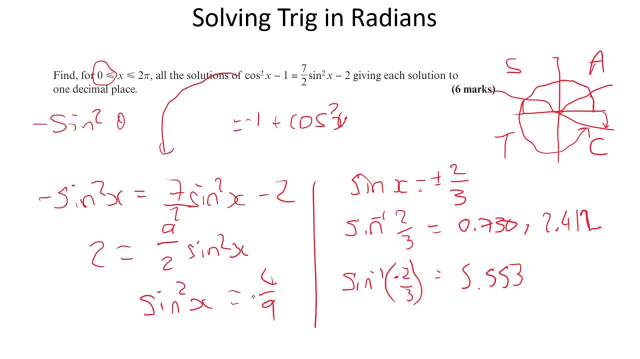 Uh, we know that because they are positive for tan and cause and therefore sign is negative. So we've got the first one. We came all the way around to this um quadrant and got this angle And we want the same distance, but we want it from pi. 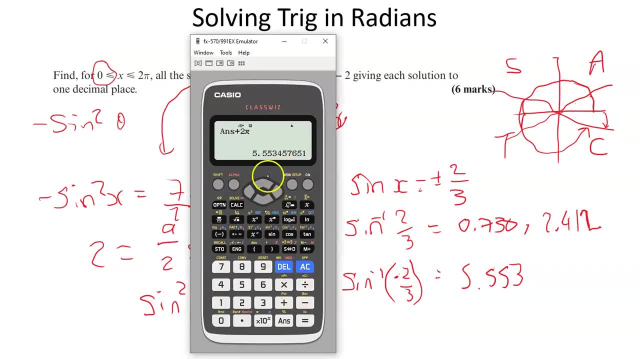 So what I'm going to do is I'm going to go back to this value here, although I want it to be positive. So I had that here. There we go. So it's that angle here that we've been working on, but it wants to be more than half the circle. 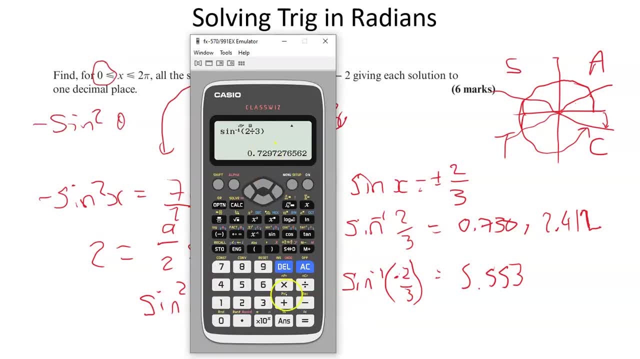 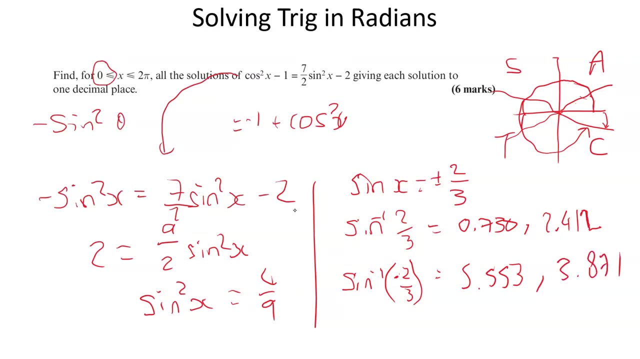 So that's why I needed it to be positive. So it's that amount plus a whole pie yet. So we have pie going there And then that angle coming around and the answer is 3.8, 7, 1.. So there are four answers to this question. 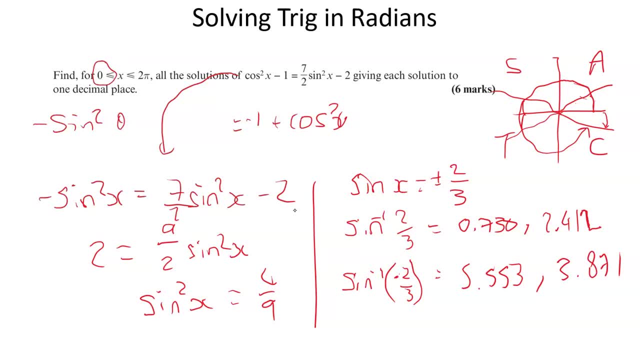 And that's uh. that's because we have this squared. We normally get two answers, but the squared uh meant that there were uh answers for the two thirds and answers for the minus two thirds. And if you think about how the graph would look, uh for sign, it would normally look like this and there'd be your two answers there. 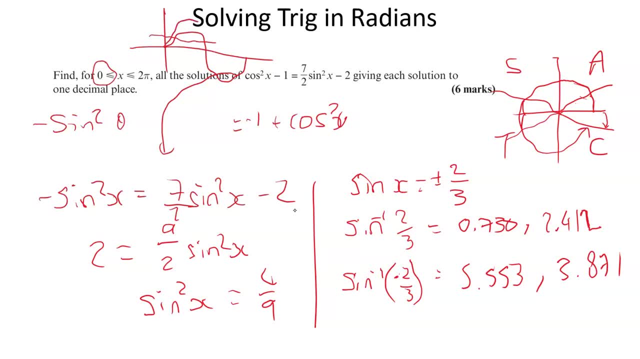 But because we've squared it, it's going to look uh. well, actually, I'm not sure it does grow, does it? It's not growing any taller, Uh, but it is going to, uh, it, probably be a bit wider and flatter. 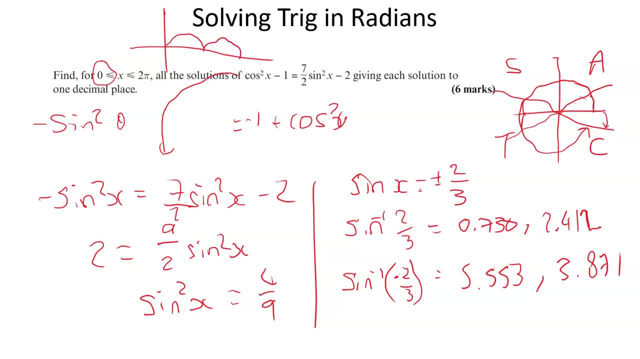 And then the second one is now positive. uh, because when you square negative numbers, they are positive. And so here you can see that there are one, two, three, four answers, and those are them in radians. But notice, I'd have done exactly the same thing if it was in degrees.